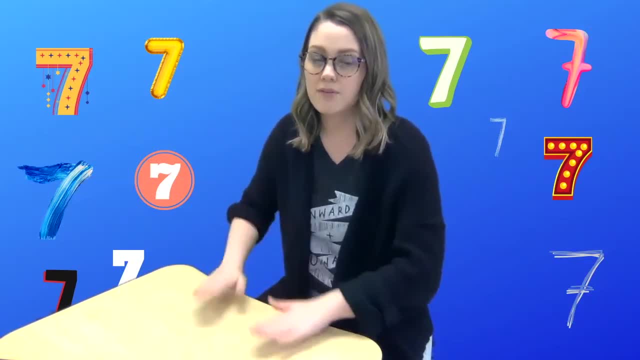 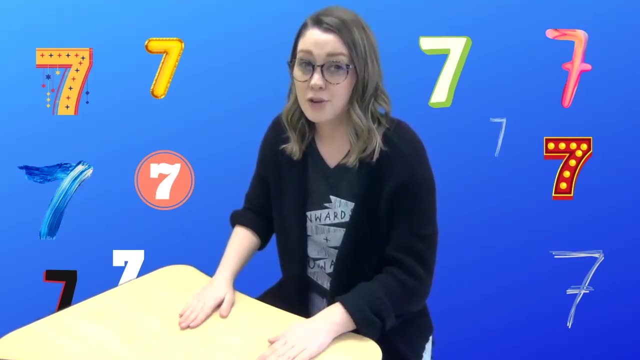 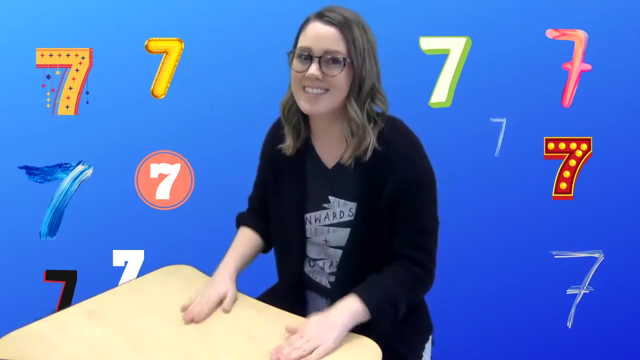 second round goes: one, two, three, four, five, six, seven. one, two, three, four, five, six, seven. The third round is a little bit harder. It goes like this: one, two, three, four, five, six, seven. one, two, three, four, five, six, seven. one, two, three, four, five, six, seven. 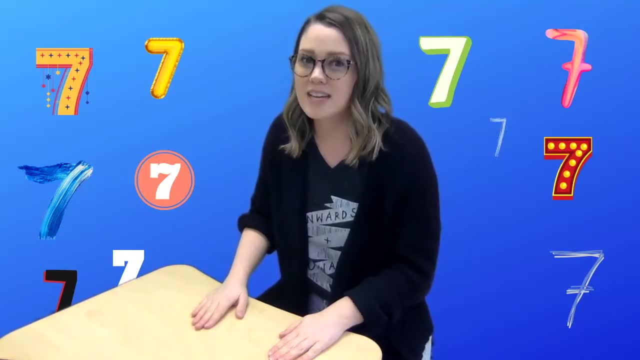 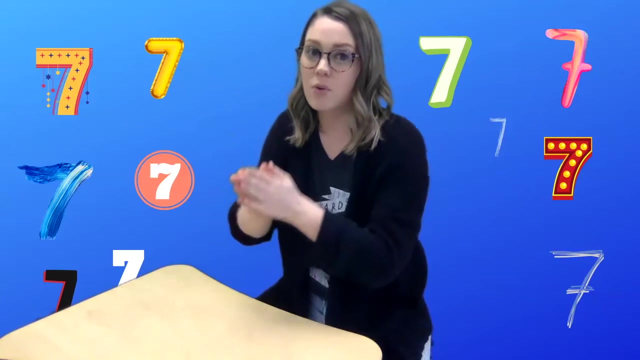 seven. you think you have that. the fourth round is the hardest. it goes: one, two, three, four, five, six, seven. so it's kind of like round three, except this time, when you get to the snap, you're going backwards. let's try it again: one, two, three, four, five, six, seven. one, two, three, four, five, six, seven. 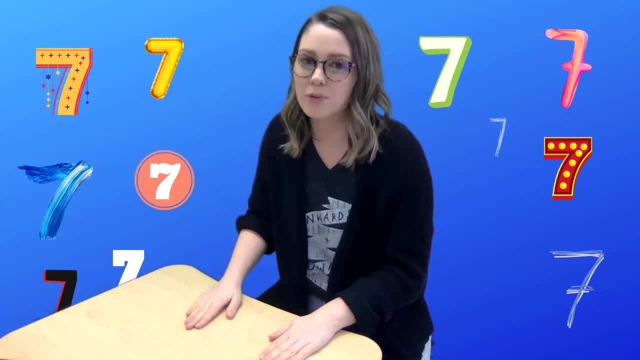 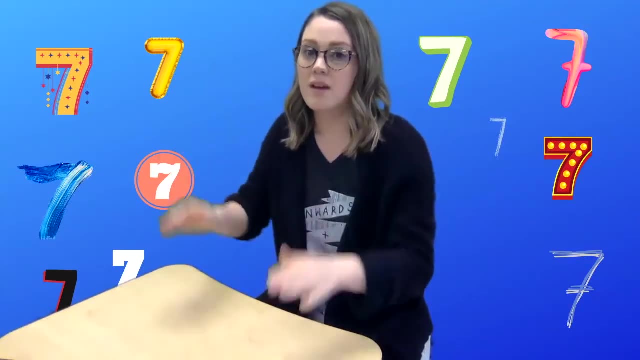 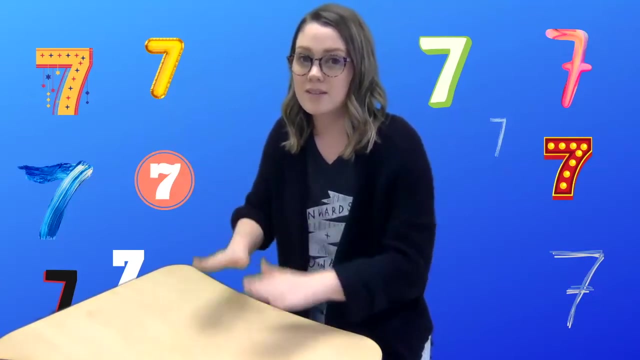 okay, and now, since we got to round four, we're gonna go backwards to round three again. one, two, three, four, five, six, seven. one, two, three, four, five, six, seven. now round two: one, two, three, four, five, six, seven. again one, two, three, four, five, six, seven, and then finally round. 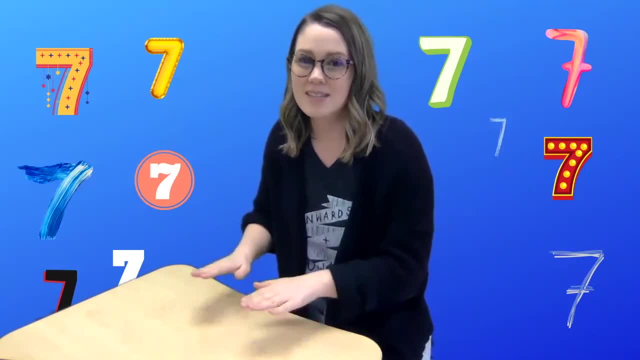 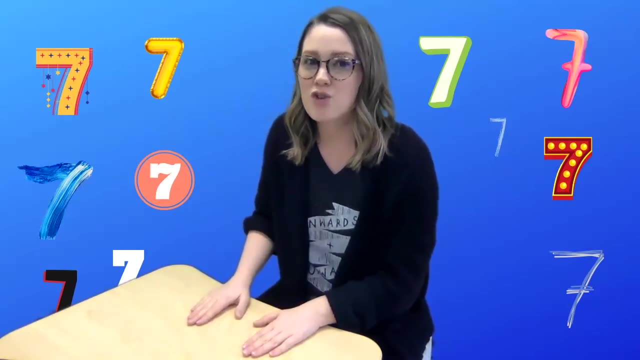 one, one, two, three, four, five, six seven. one, two, three, four, five, six seven. now that you have it, we're going to try to play a little bit of a game with you and we're going to play a little bit of a game with you. and we're going to play a little bit of a game with you and we're going to play a. 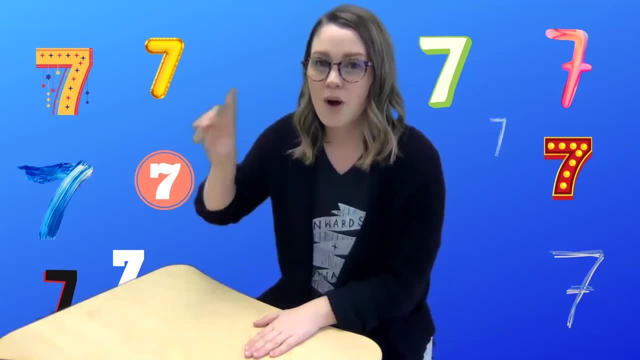 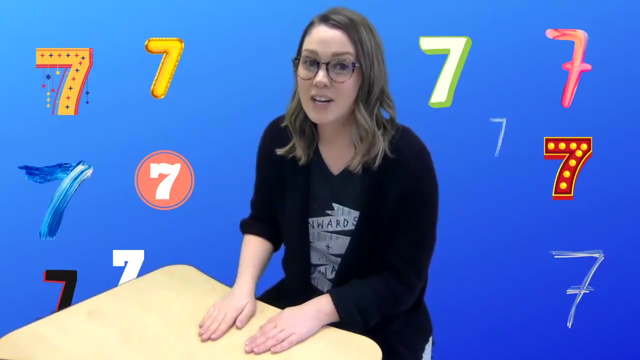 little bit of a game. we're going to do the rounds three times in a row. the first time we'll try pretty slow, the second time we'll go medium speed and then the third time we'll see if we can perform this fast. finally, at the very end, i'll give you a challenge. are you ready? here we go. one, two, three. 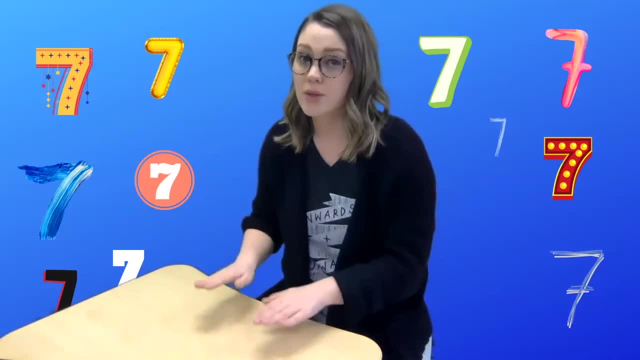 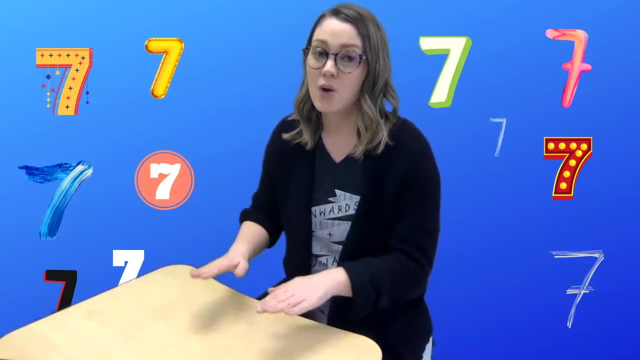 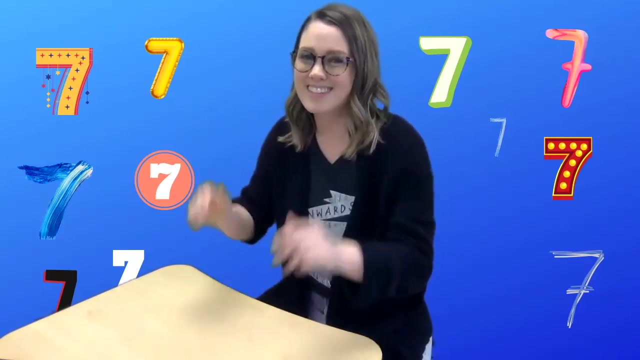 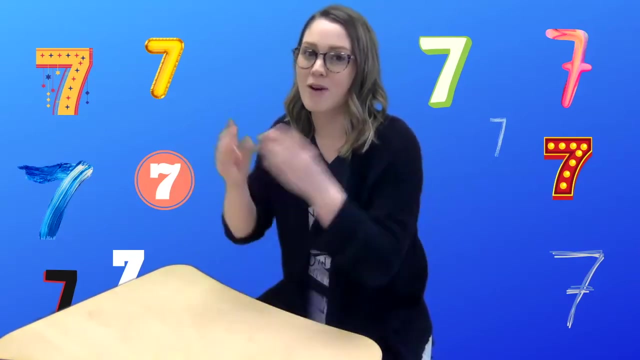 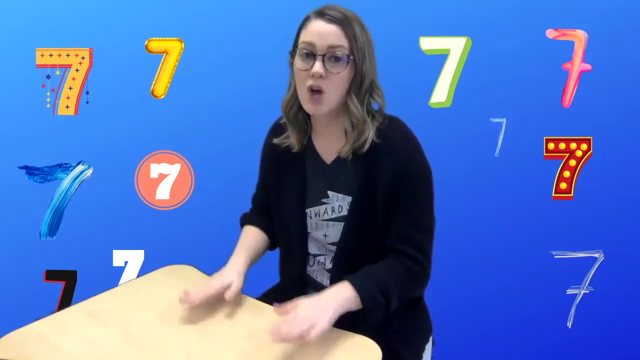 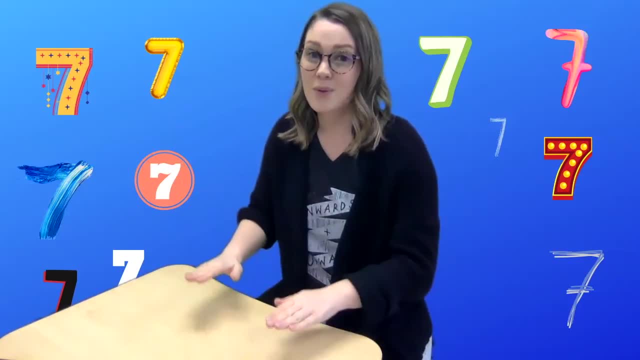 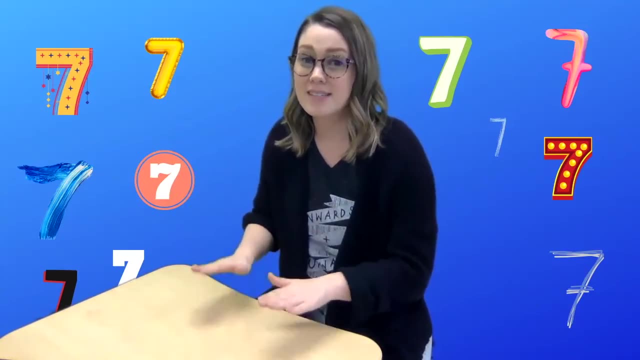 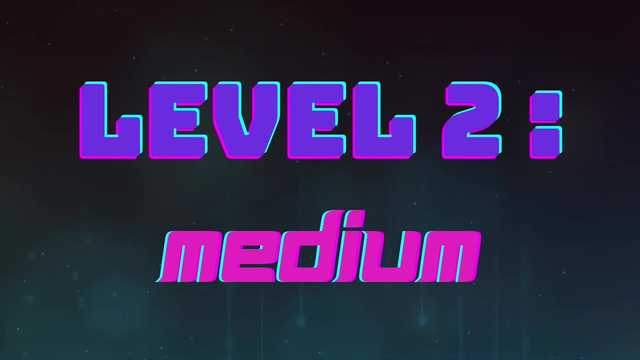 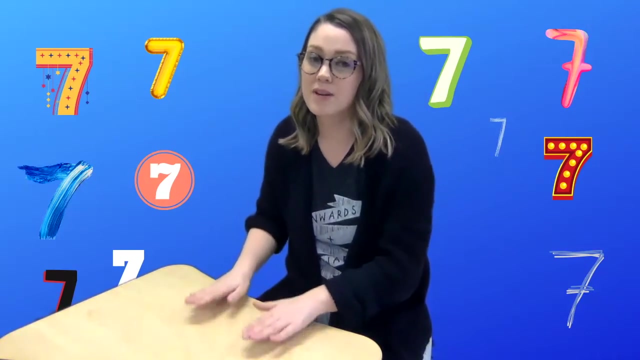 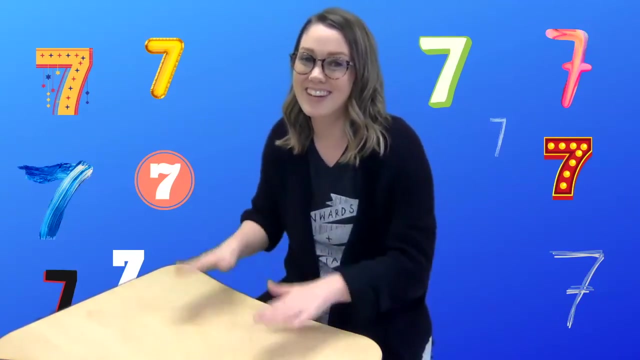 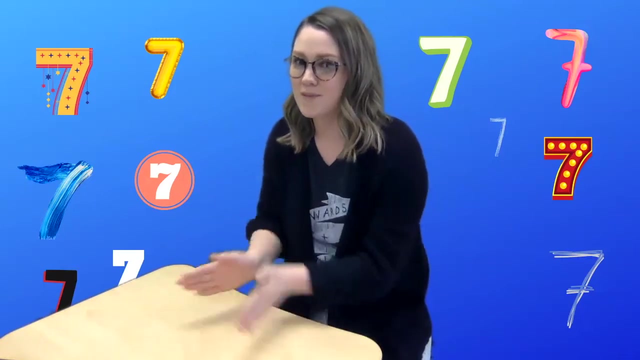 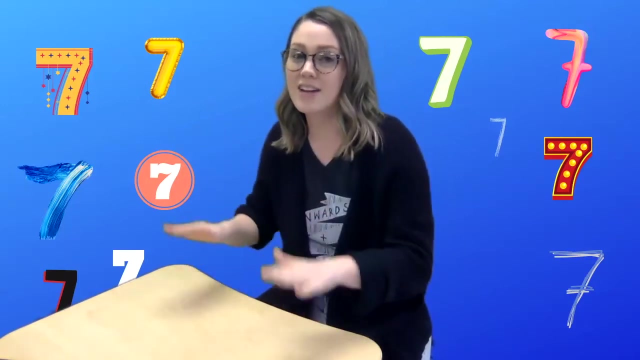 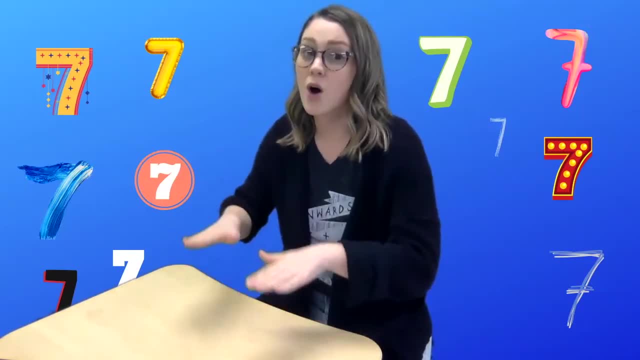 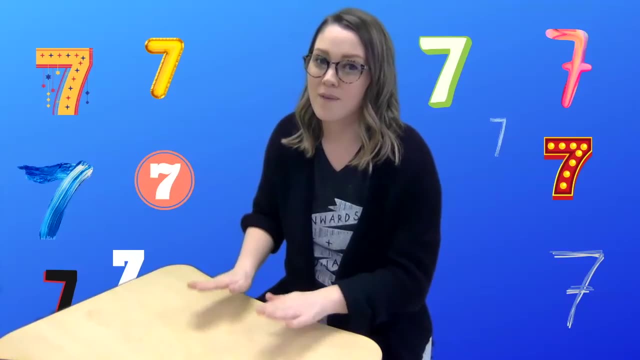 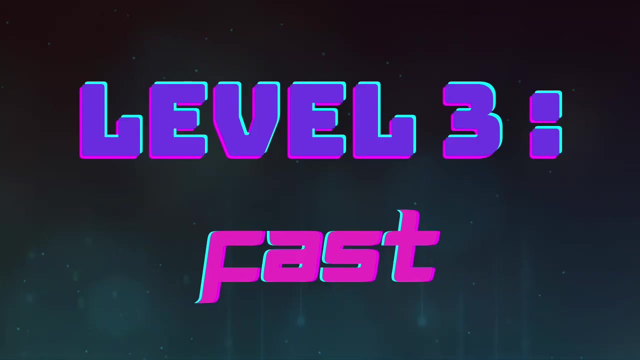 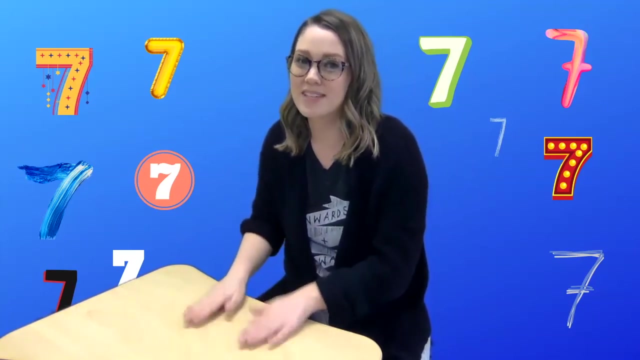